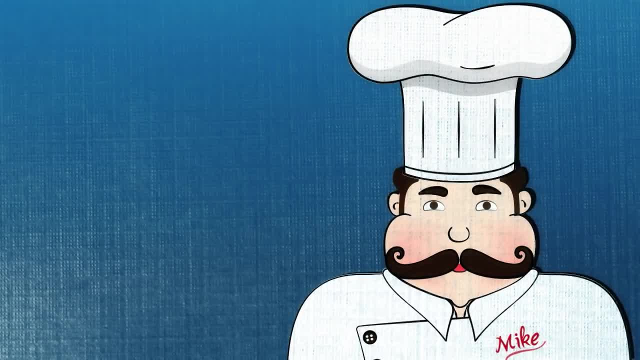 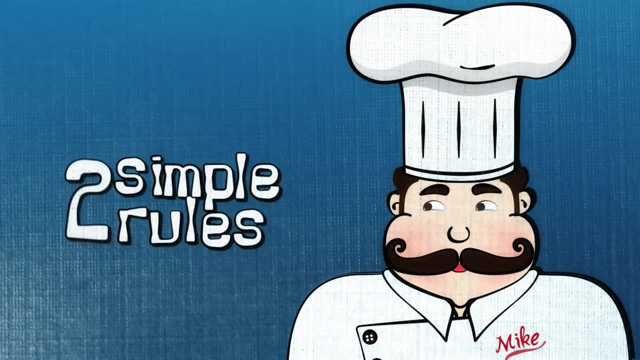 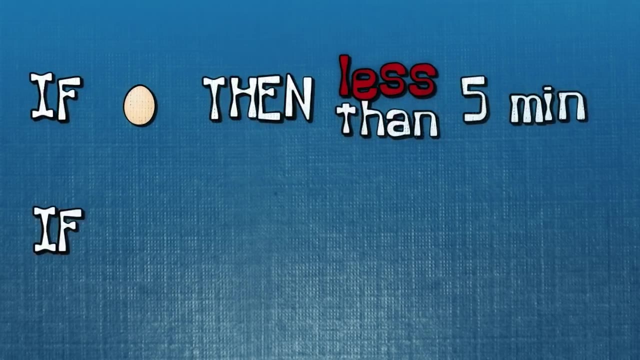 ask her best friend, Mike, who is a chef, for some tips. Mike noticed that Jane's robot didn't consider the egg size when deciding the boiling time, so he gave Jane two simple rules to follow. If the egg size is small, then boil for less than five minutes. If the 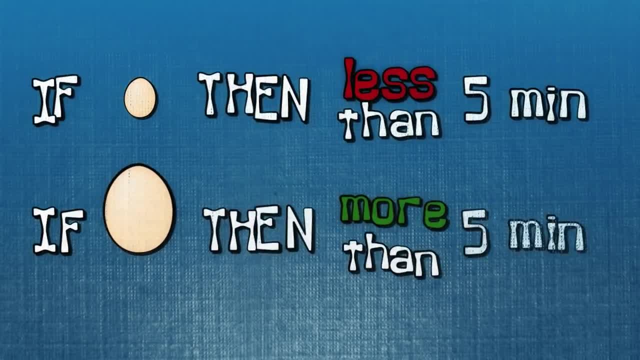 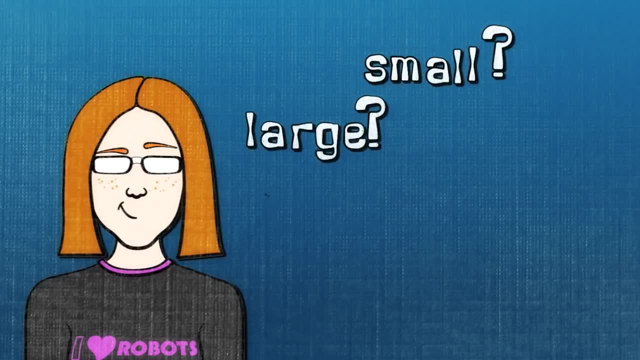 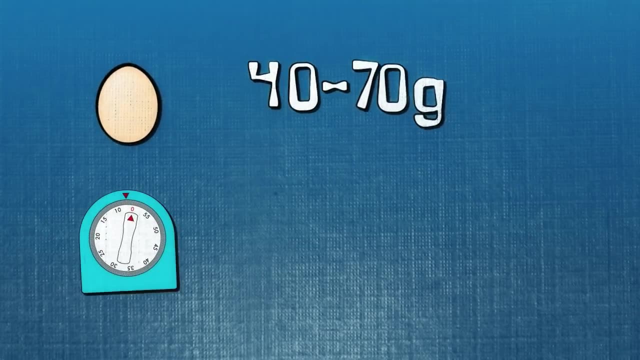 egg size is large, then boil for more than five minutes. But Jane thought… What does small, large, less or more mean? We know that egg weights can range from 40 to 70 grams, with boiling times ranging from 3 to 6 minutes. 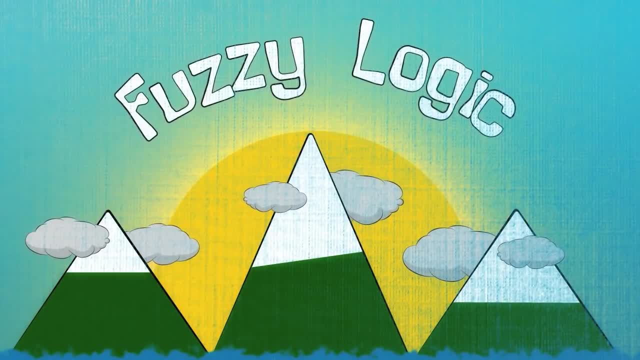 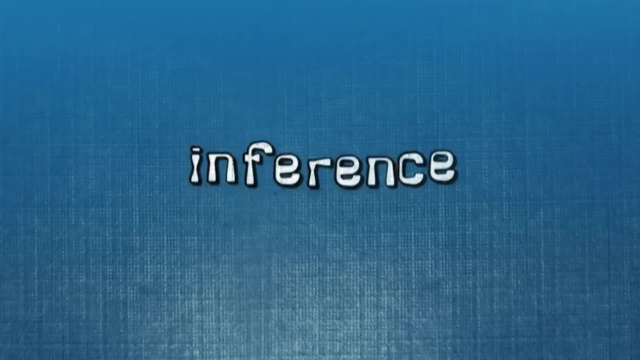 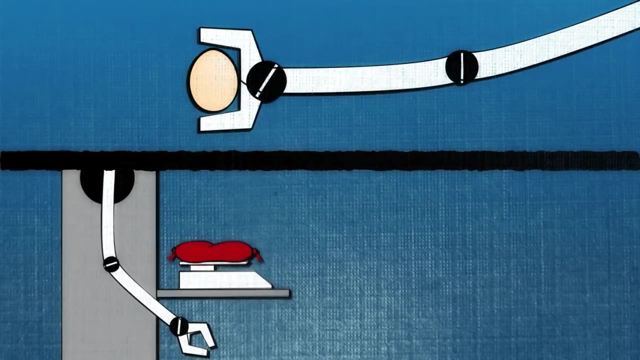 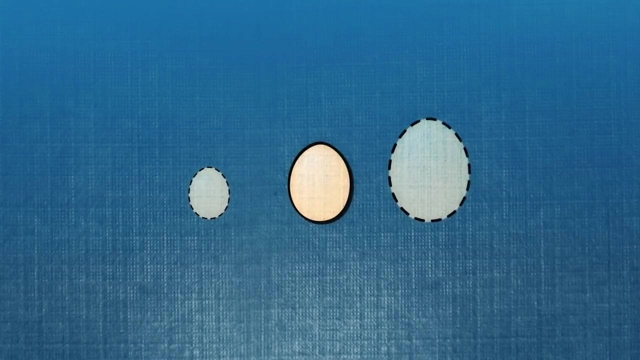 Fuzzy Logic utilizes this knowledge. Designing the intelligent egg-boiling robot requires three steps: Fuzzification, inference and defuzzification. Step 1. Fuzzification: The robot takes an egg and measures its weight. According to fuzzy logic, any egg is both small and large, but to different degrees. 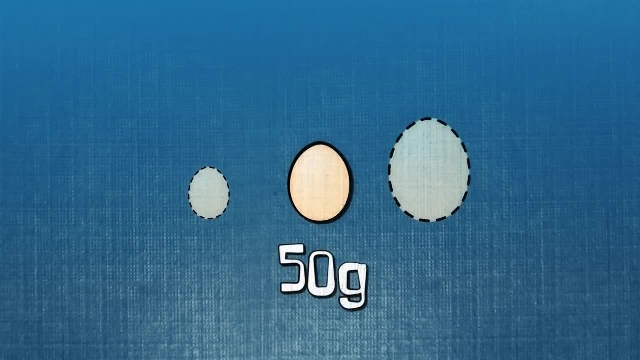 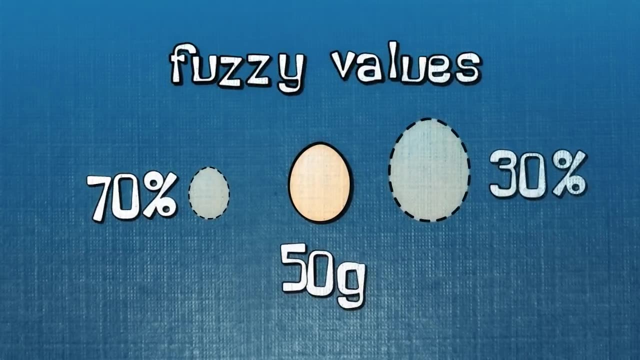 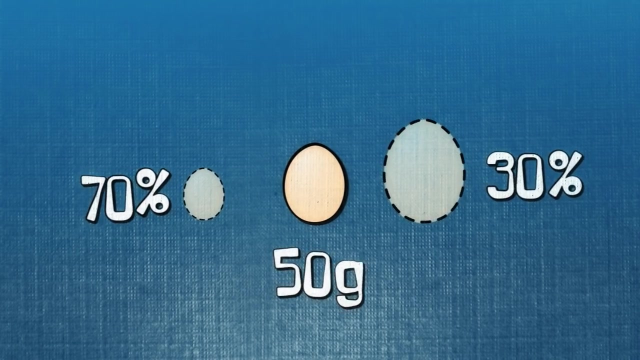 For example, our robot considers a 50 gram egg as small in a larger degree and as large in a smaller degree. Those are called fuzzy values, Step 2. Inference: Since the egg is both small and large in different degrees, the robot applies Mike's two rules, but again in different degrees. 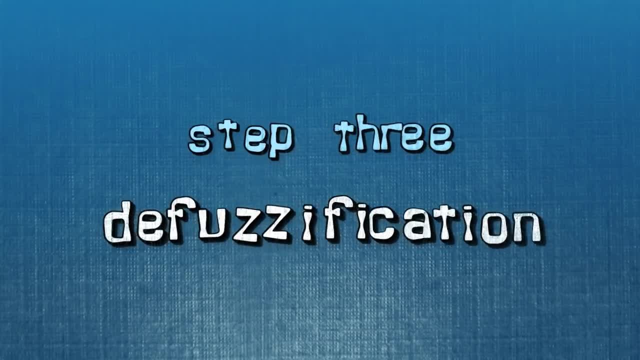 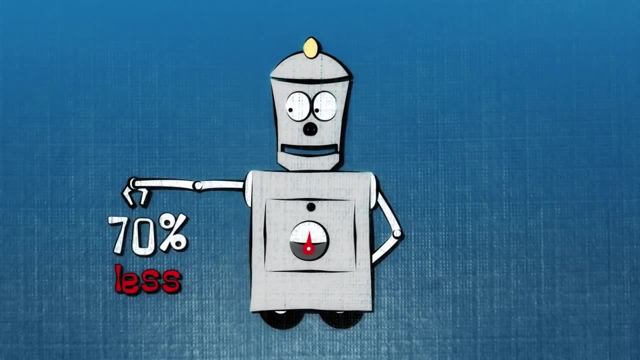 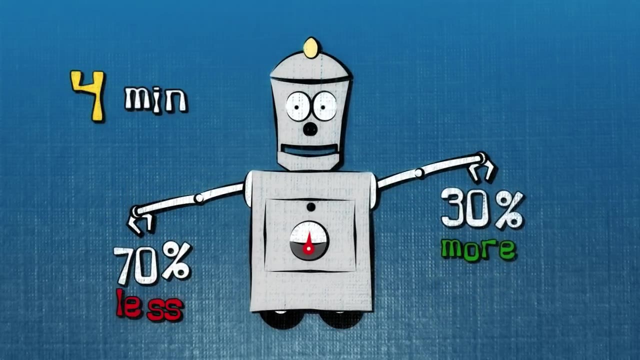 Step 3. Defuzzification. The robot must now calculate the actual boiling time based on the fuzzy values from the previous step. Hence, for the 70% less and 30% more than 5 minutes boiling time, a balanced decision would be to boil the egg for 4 minutes. 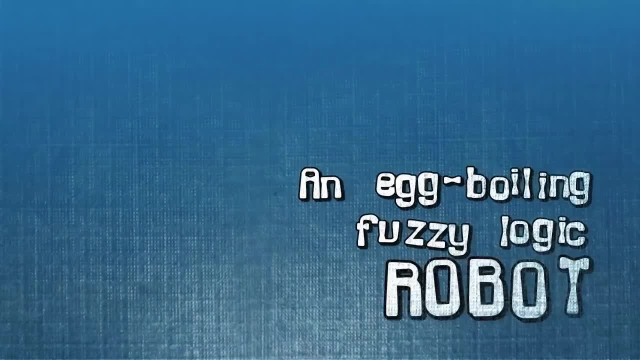 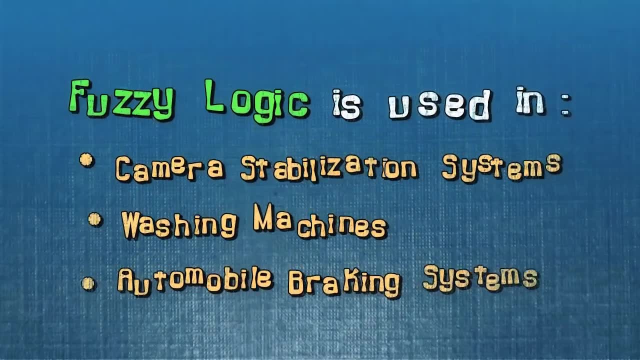 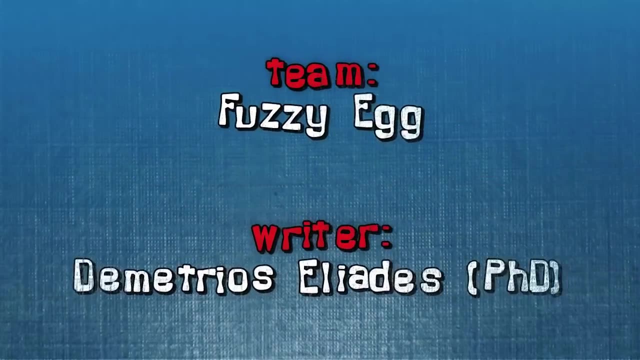 Our intelligent fuzzy logic egg boiling robot is now ready For more information. visit our website at www. whereverfuoziescom. To learn more. visit our website at wwwwherefuoziescom. More info on our website: wwwwherefuoziescom. 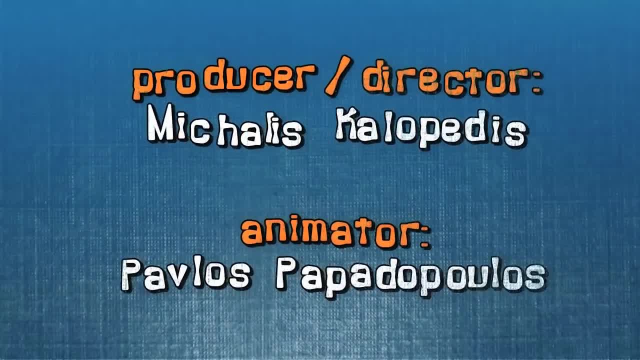 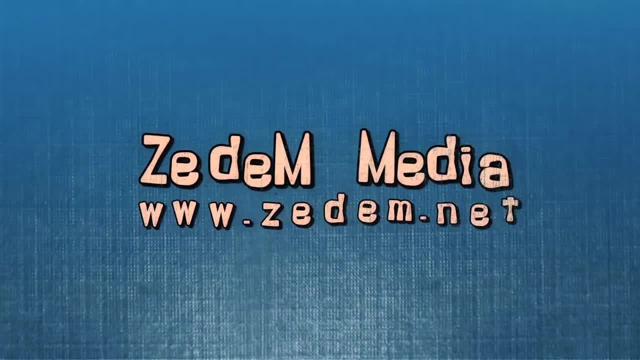 More videos. Subscribe to our YouTube channel. Click on the bell icon to be notified of our new videos.